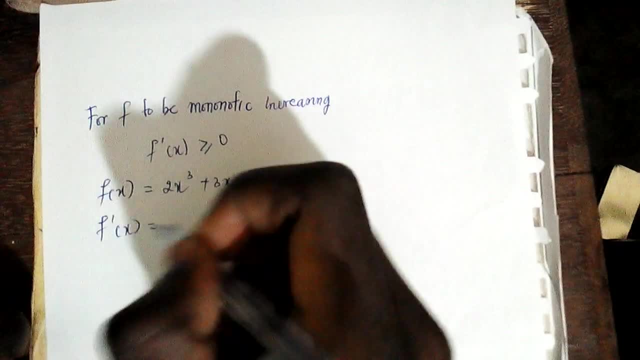 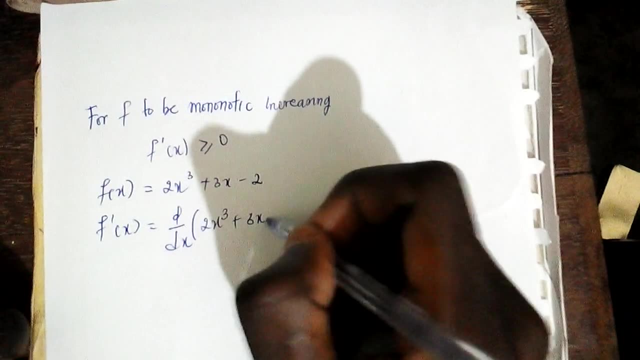 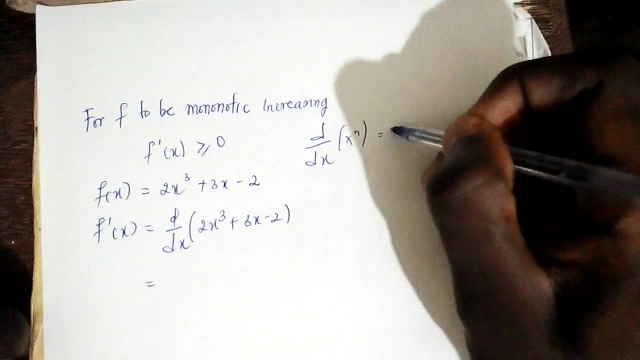 So I need to look for the first derivative. So the first derivative is just gotten by differentiating my function one time with respect to x plus 3x minus 2.. So generally if I differentiate the function x to the power n, I drop the power. I take x raised to the power n minus 1.. 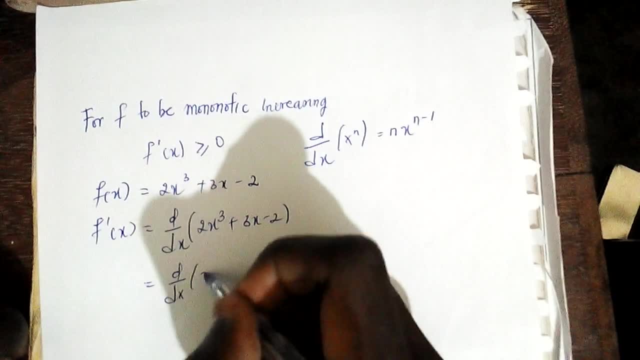 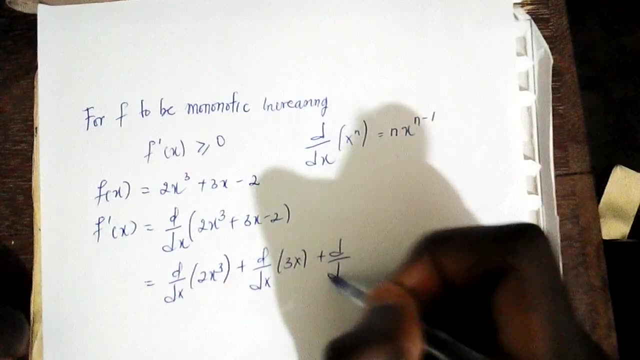 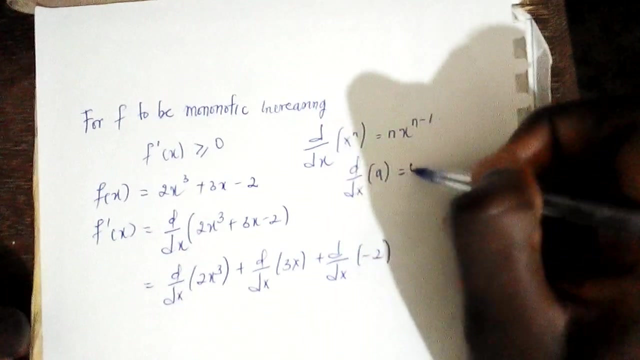 Alright, so this is the same as the derivative of 2x cubed, plus the derivative with respect to x of 3x, plus the derivative with respect to x of 3x With respect to x of negative 2.. Now, standardly, whenever I differentiate a constant with respect to x, I get 0.. 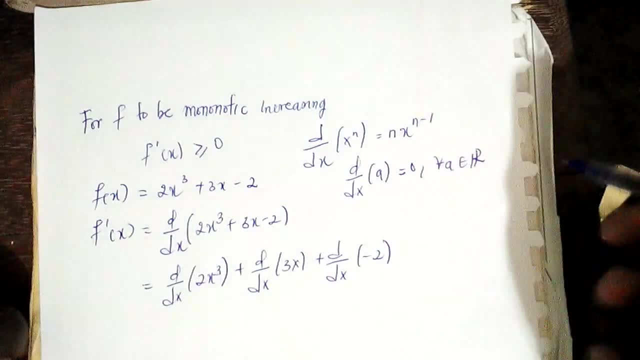 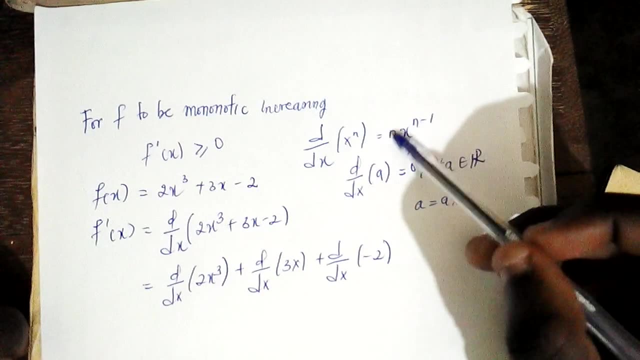 So a is in the set of real numbers. Why? Because this constant a can be written as a x raised to the power 0. So when I differentiate, the power is 0.. So when you drop the power, the n becomes 0. 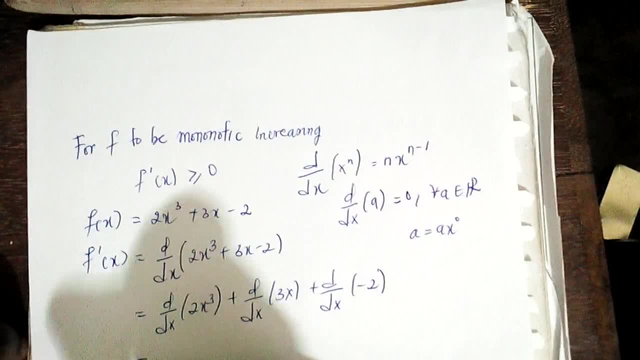 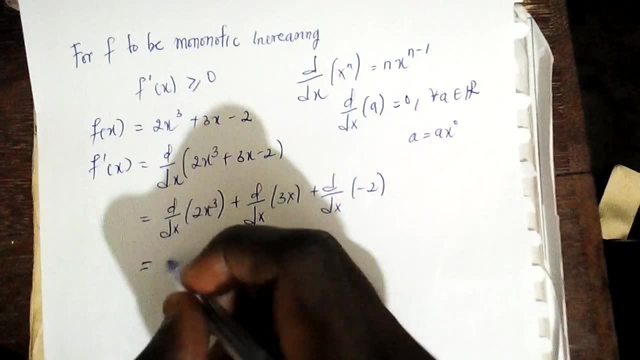 It multiplies with anything, you get 0. Alright, so our first derivative in this case is going to be: So the first derivative is going to be: When you differentiate this, you have your 2 outside. it's a constant. 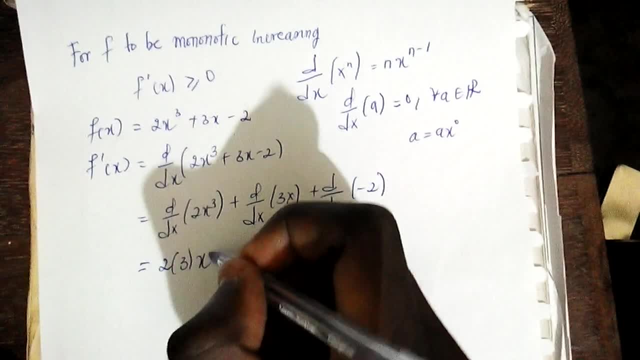 When you drop down the derivative, it multiplies with a 2.. Then you have x raised to the power 3 minus 1, which is 2.. Plus you keep your 3 outside. it's a constant. When you differentiate the x, you just get 1.. 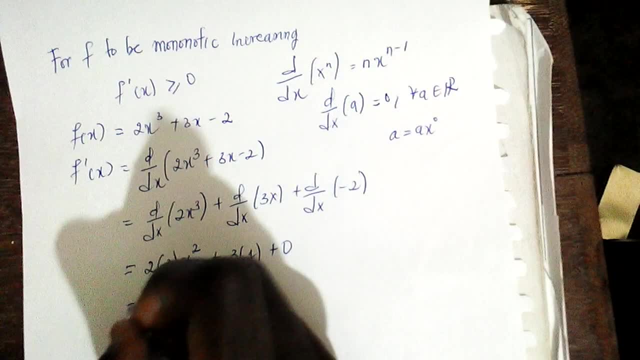 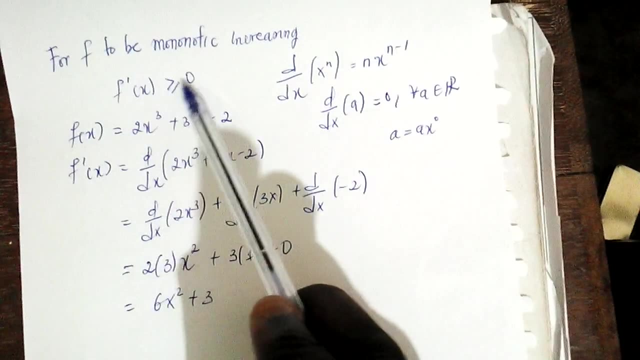 Then plus, when you differentiate the constant, you get 0.. Alright, so this gives you 6x squared plus 3.. Now the aim is to show that f prime of x is greater or equal to 0. So here is how we post it. 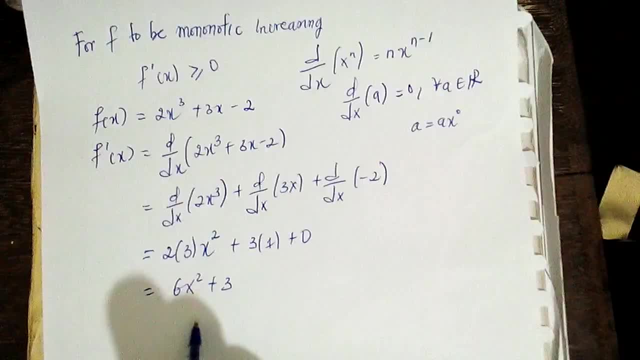 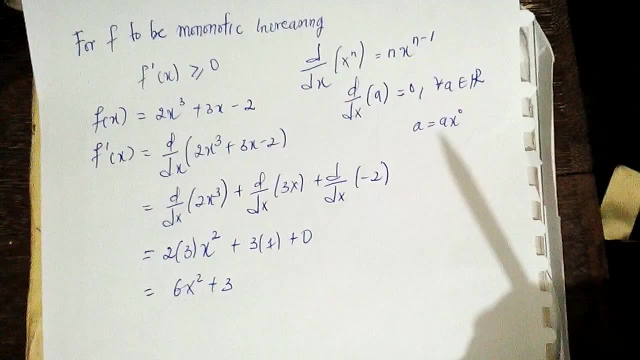 This is our f prime of x, So we need to now justify that this f prime of x is greater or equal to 0. Either greater than 0 or equal to 0, or greater or equal to 0.. Okay, so clearly, for all values of x in the set of real numbers, right. 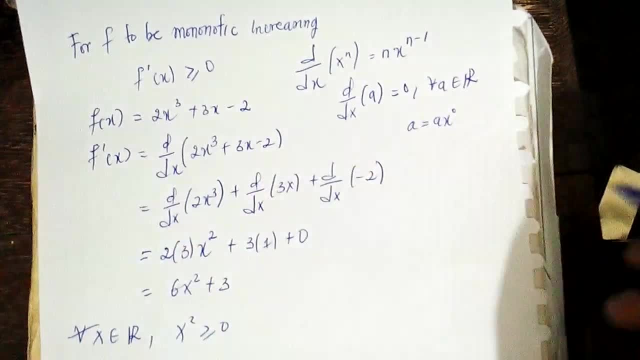 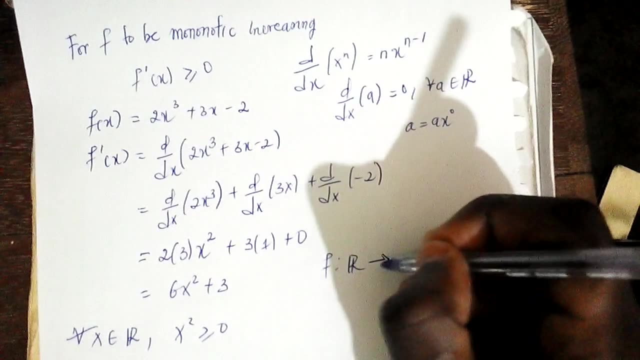 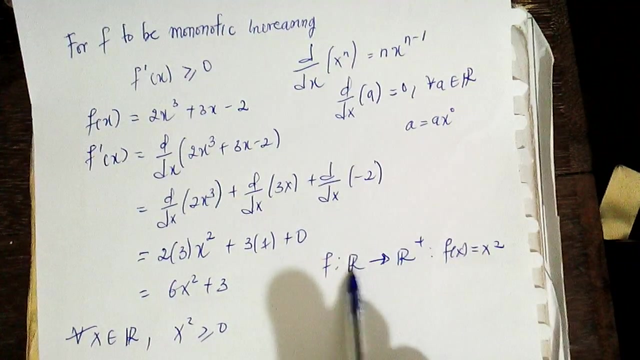 we have that x squared is greater or equal to 0 whenever it's squared in number, Because the function is from r to r plus, That's the function f of x. It's equal to x squared. The domain is r and the co-domain is: that's: the range is r plus.